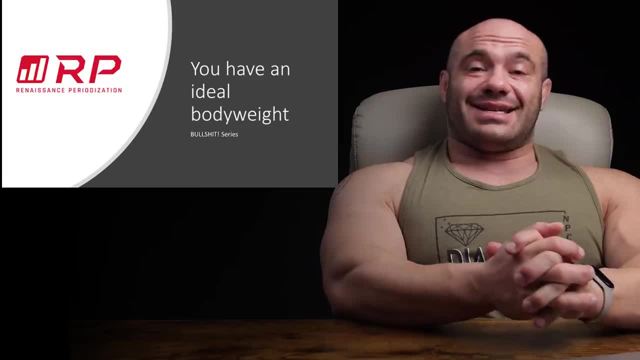 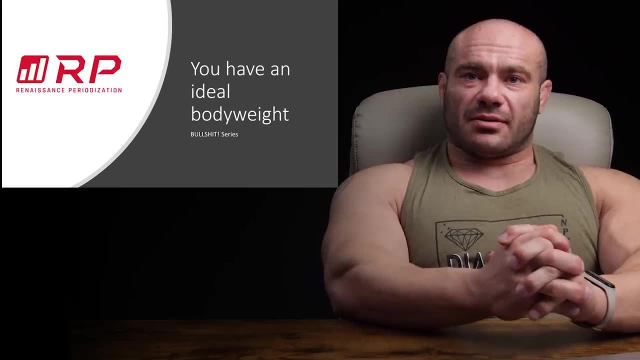 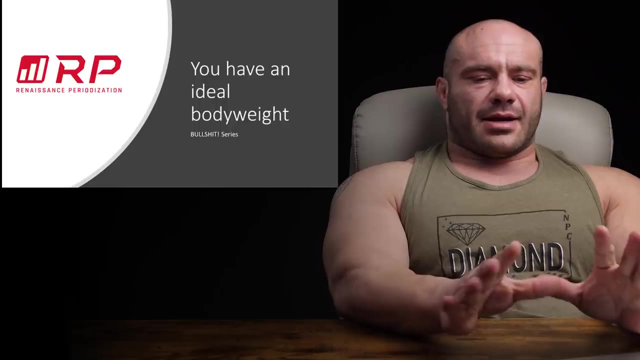 Hey folks. Dr Mike here for Renaissance Periodization and the idea that you have an ideal body weight that you should be striving for is bullshit. It's not true. Stop it. Okay, world's worst Arnold impression. tell us actual facts. Here's the deal. The idea of an 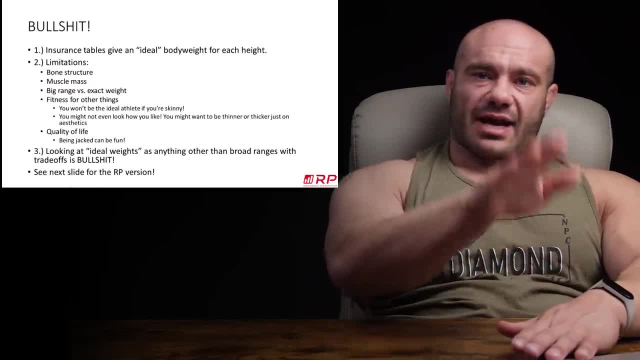 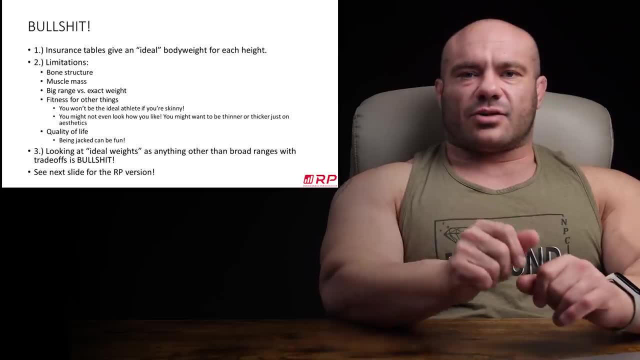 ideal body weight comes mostly from insurance tables. These are tables of heights and weights and basically, if you're 5'11 and you're a male, you should weigh xyz amount of weight according to these tables, and the way they're derived is usually from just indices of who lives the 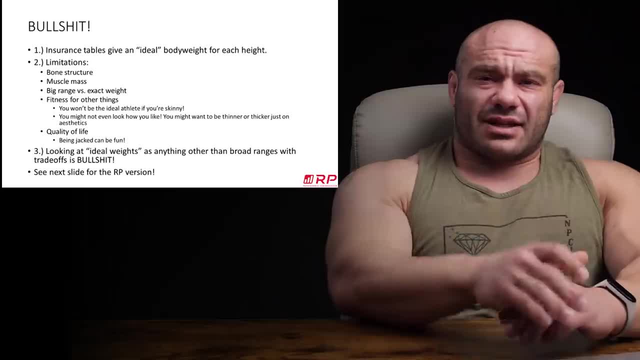 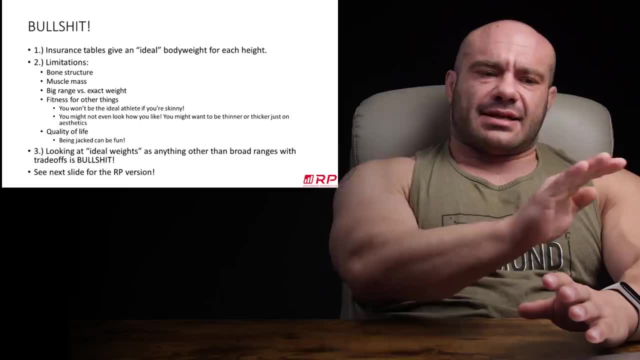 longest. So they're based not even on health, but on longevity, which is a very, very good proxy for health. not exactly the same thing. And what they did, these insurance companies, is they didn't manage to do a whole lot of data analysis. They did a ton of data analysis on the back end. 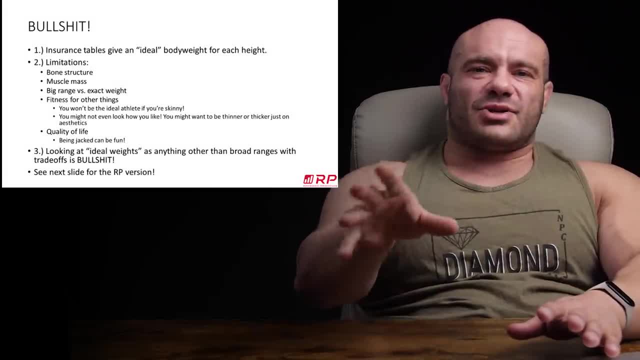 but on the front end they didn't really put out back in the day a normal distribution that says: well, here's the average healthy body weight for people that are 5'11.. They just did the average healthy body weight for people that are 5'11.. They just did the average healthy body. 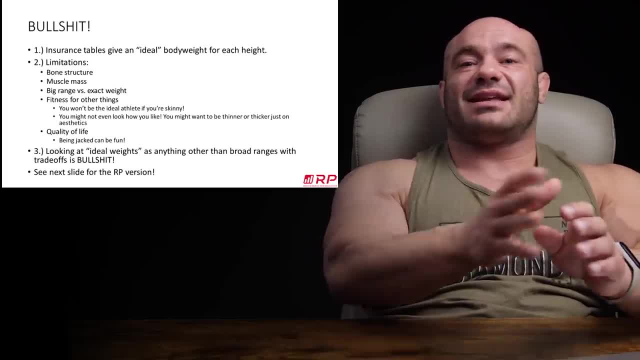 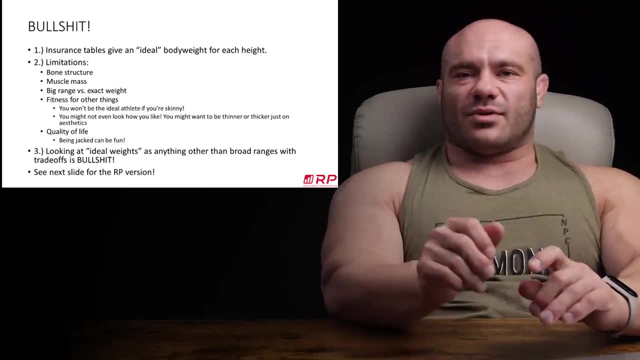 the average and only reported. They didn't say what the standard deviation was. They didn't say that a lot of other values close to that are basically undifferentiably healthy and prone to making you live a long time. That's just one of the limitations. Let's talk about a few others. 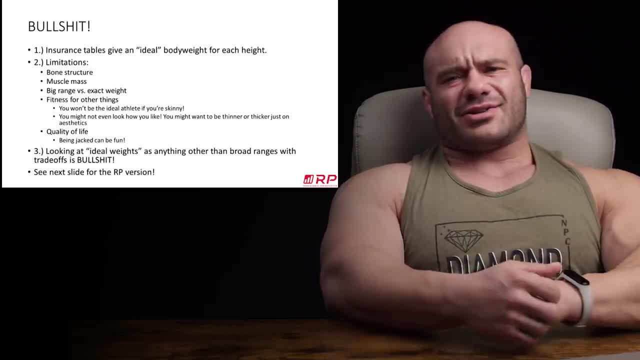 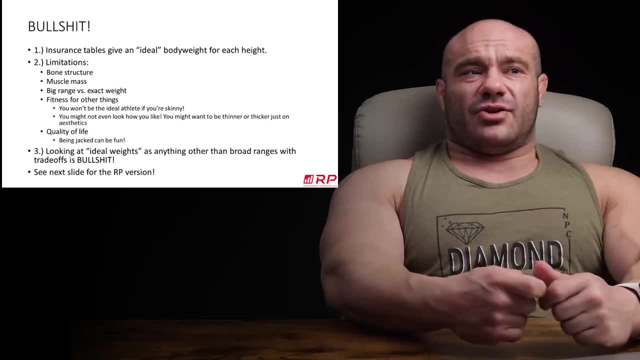 So bone structure. If you're a 5'11, congratulations. Unlike me, you actually got to be an adult height. You're 5'11.. If you have thick-ass big bones, you may need to weigh a lot more in order to not be. 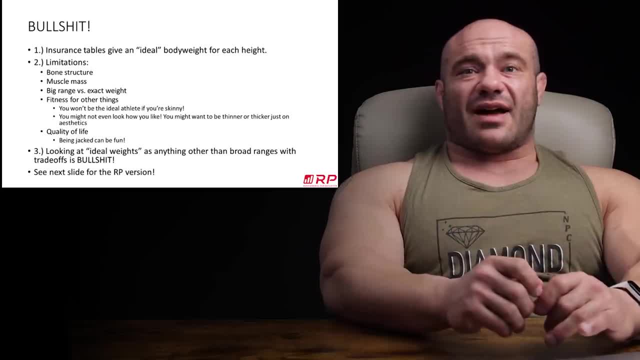 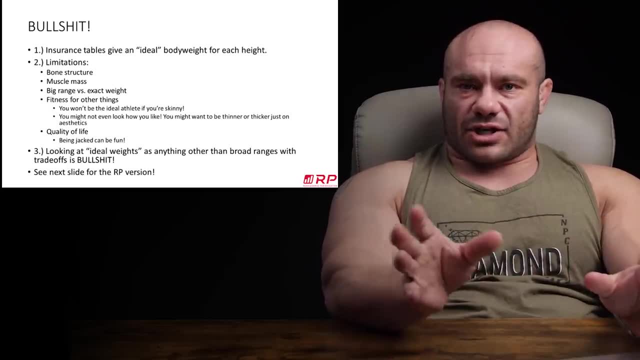 an unhealthy compared to a person with really small bird bones that at 5'11, they could weigh very, very little and still actually appear and be very healthy because they just don't have a lot of bone mass, not a lot of tissue to put on those bones etc. So bone structure matters, which is 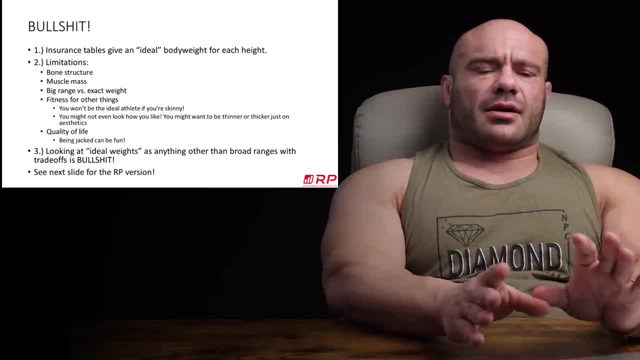 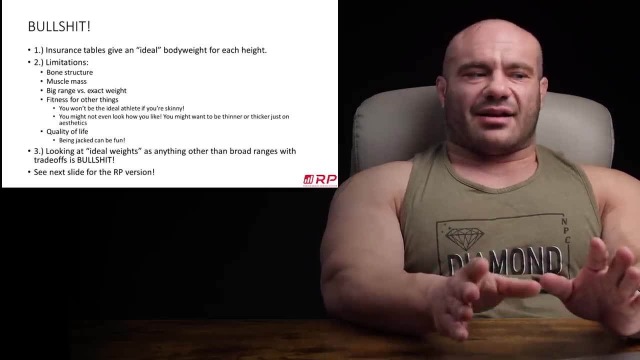 why you can't just have one ideal weight without knowing your own bone structure. Usually, when you look up ideal weight on the internet- which is how most people do it- and say I have to weigh 120 pounds, there's no calculator for bone mass or anything like that. Another problem is muscle. 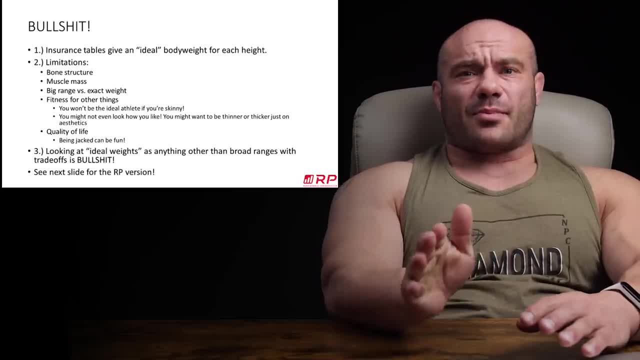 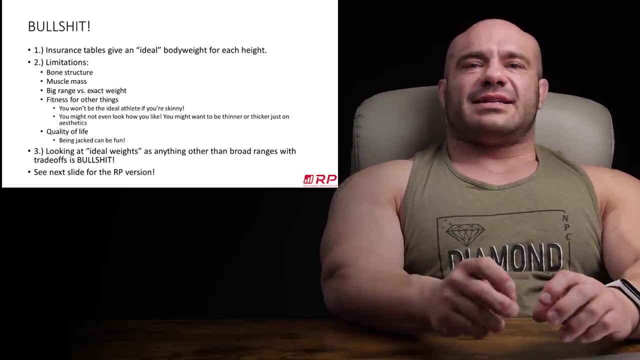 mass. You can have a lot of muscle mass and up to a pretty high point. You can have a lot of muscle. you're very healthy and can live a super long time with a lot of muscle. that doesn't count for that. Most of these things were. these indices were derived in the 30s, 40s and 50s And back. 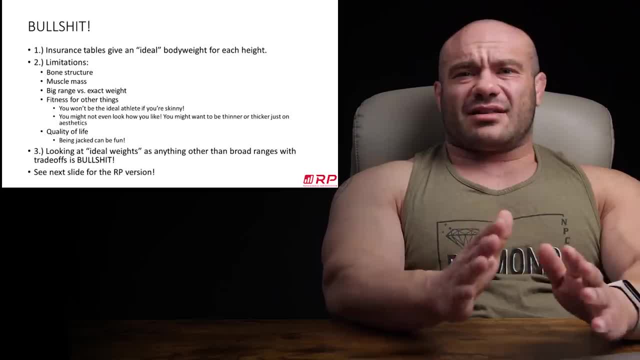 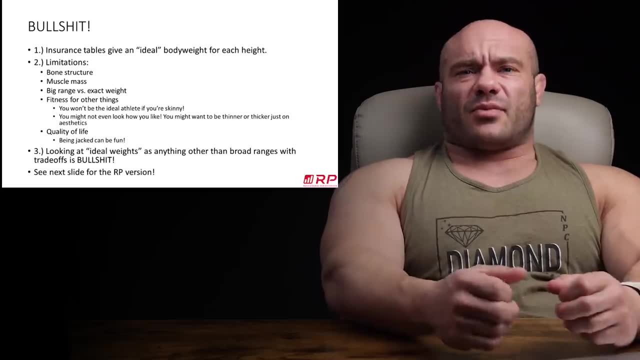 then most people didn't train and muscularity was just something that was genetically varied or varied according to your job, Like if you were a dock loader. maybe you were slightly more muscular, marginally more muscular, but people weren't really super jacked. Nowadays, a ton of people work out and the insurance tables just absolutely don't cover them. For example, some of the CrossFit girls that are at the top of the world for the sport. they're like the damn near forever, but they're considered overweight and obese, sometimes on these tables. 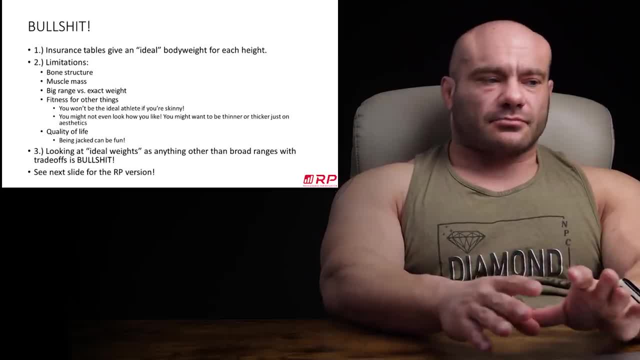 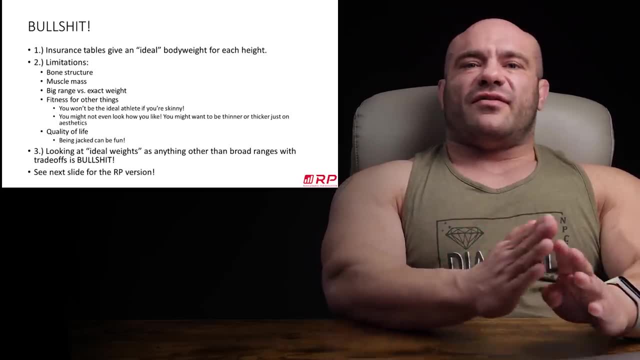 because they're just never met with muscular people intended. Another thing, something I already mentioned, but it bears repeating: There is a range, a very large range, of very healthy body weights for any given height. The insurance tables just give one number and it's usually in. 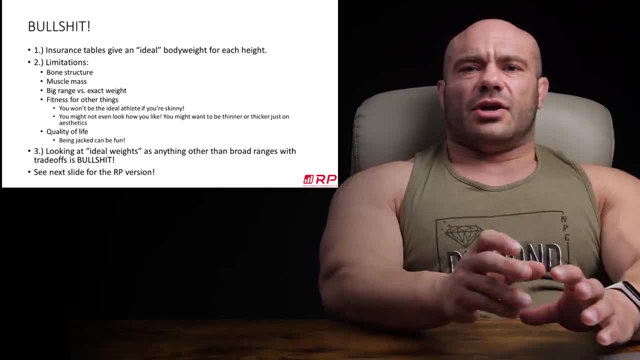 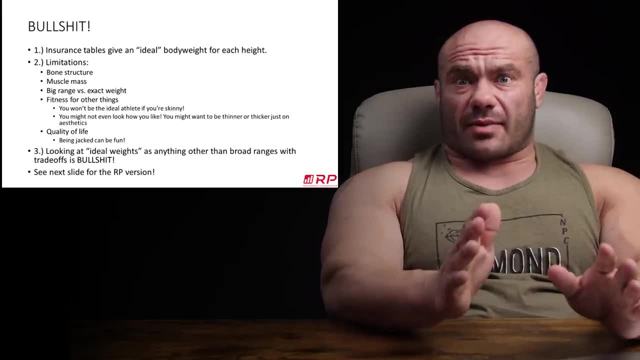 the middle or lower end of that number and it doesn't cover that whole range at all. So if you're thinking you're 150 pounds and you're like, ah, I need to be 137 in order to to be, that's my ideal weight, It's my ideal. People talk about all this all the time- Talk. 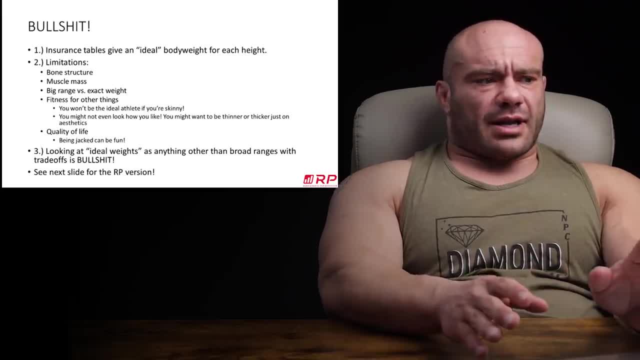 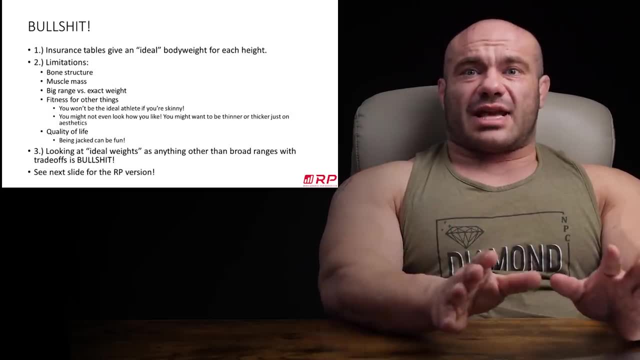 about their ideal weight. Well, hold on a second. Given that you're in that range, it could actually be that 150 pounds, health-wise, is statistically undifferentiable on a large scale from 137 pounds. So your journey to your ideal weight is already over. You're there, Congratulations. You just had. 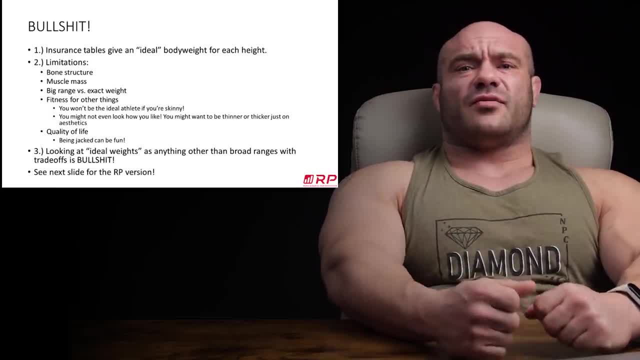 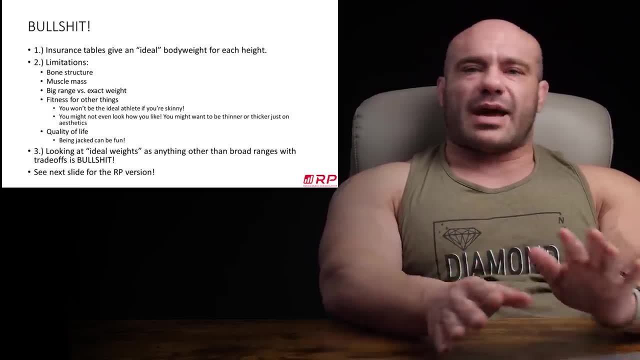 no idea And you're like trying to lose the 13 pounds and it's fucking annoying because you have bigger bones and a bit more muscle. It's really annoying because you're ultra lean down there and way too lean and you're bad sleep and bad hormones- all sorts of stuff No one ever told. 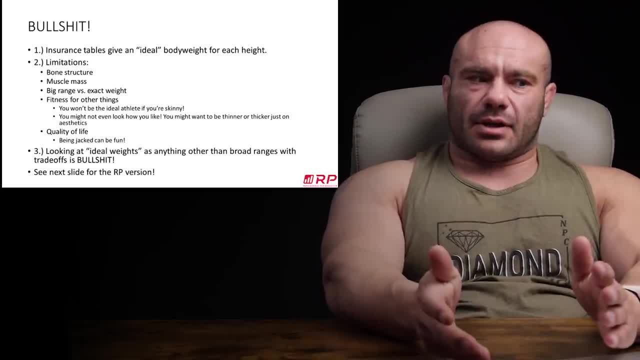 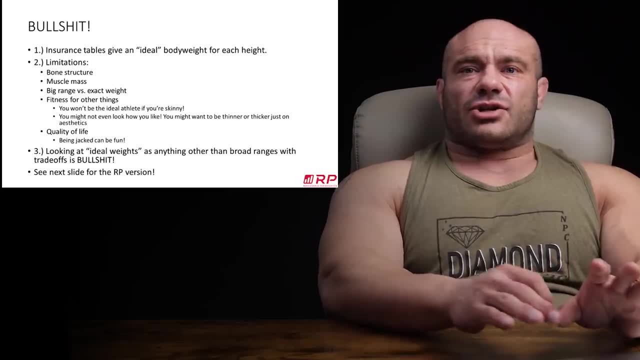 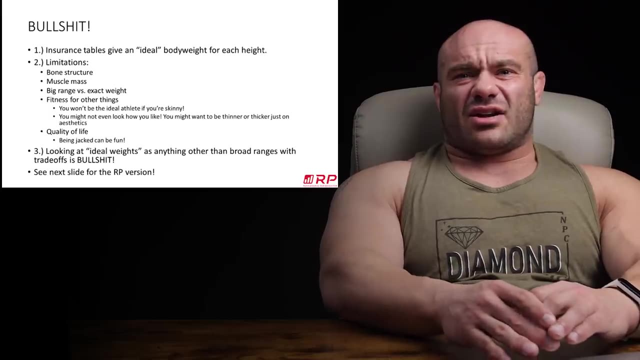 you: Hey, there's a range and you're already in that range, You already won. Another thing is that fitness for other things is a consideration that the insurance tables for ideal weight never really check. So like you can be your ideal weight, but you're like a skinny guy or skinny. 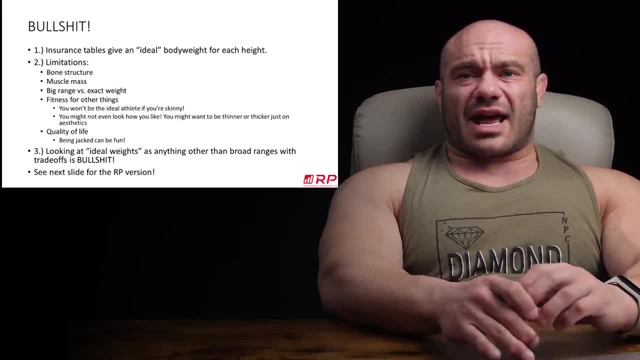 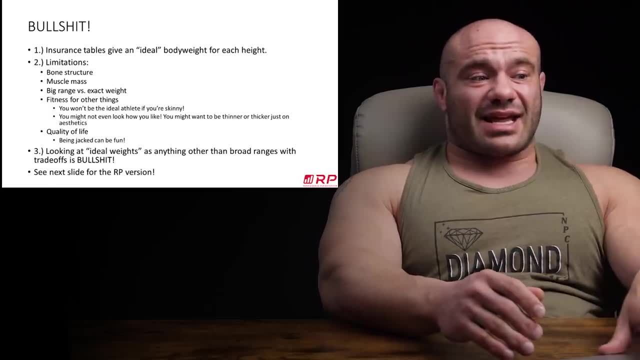 girl from the fifties. Like: what the fuck sports are you going to be good at? If you want to be good at physique sport, if you want to be your Jack power lifter or a strong woman or play ball or soccer, this shit doesn't take any of that into account. Like, yeah, if you want to be a 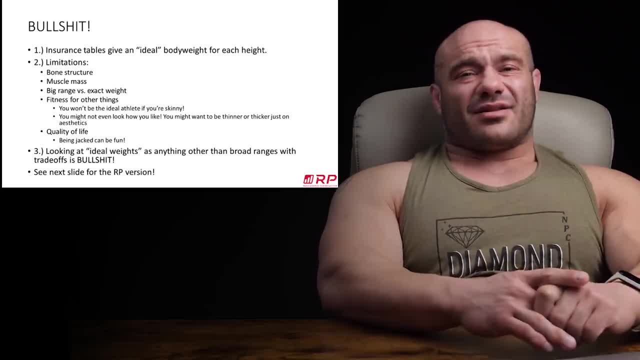 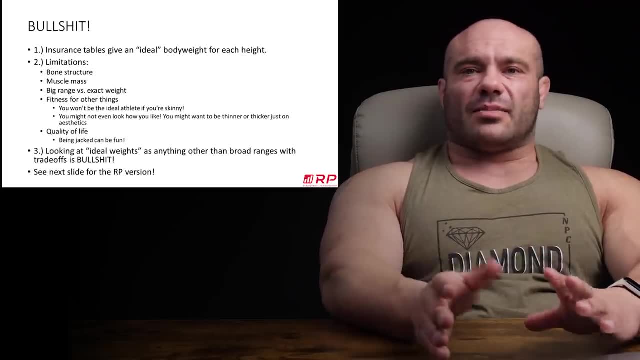 skinny, useless motherfucker. an ideal weight is kind of sweet, But other than that, your sport can determine your weight. Sometimes it's below the ideal weight, Sometimes that's at it very close, And sometimes that's well above. all of those are healthy, but some of those are just. 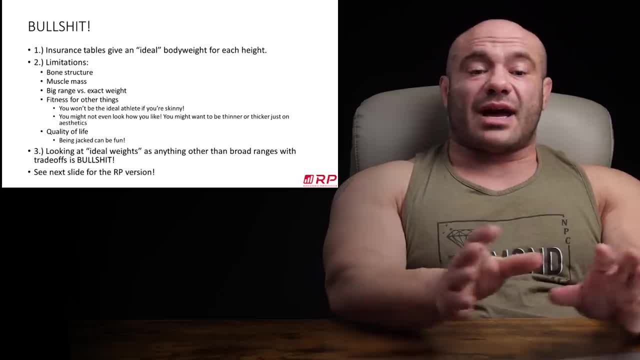 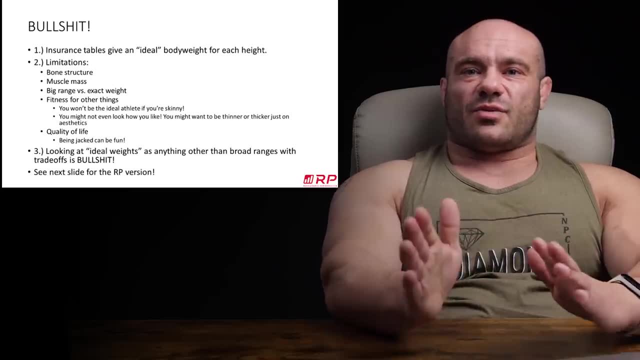 better at the sports you chose than others. So when you're making a decision of what body weight should I be, Yeah, you can look at the ideal range just to know what it is, but also make sure that you choose the ideal weight for your sport If you actually want to be good. 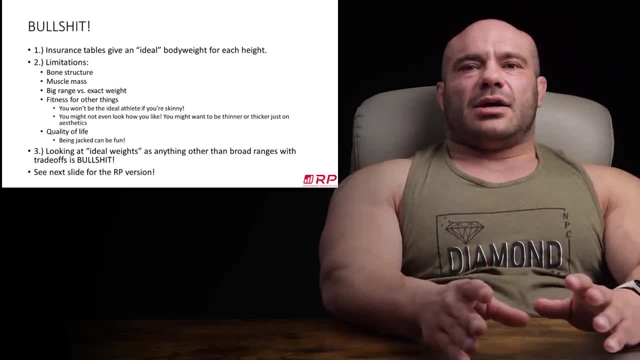 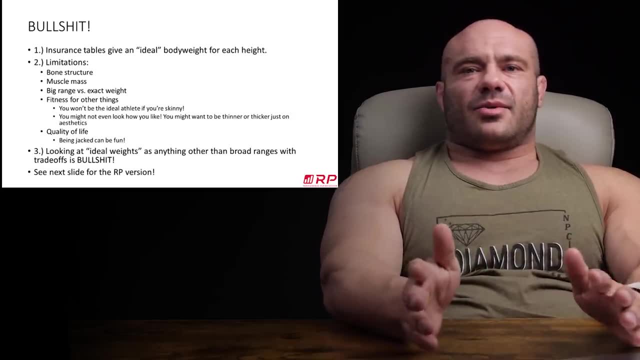 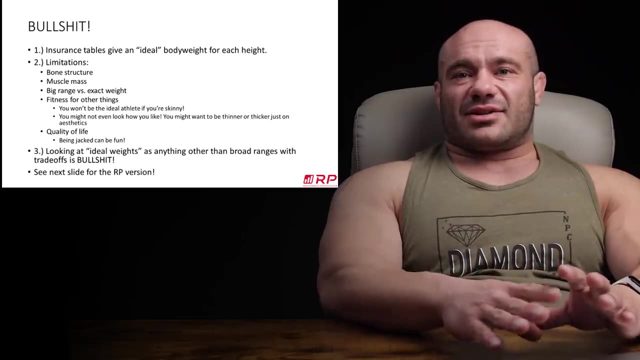 and what about aesthetics? You can want a thinner look And this is something that, with political correctness, as nasty as it is, is be one of the- probably one of the, I don't know. first, evidence-based people. to say this out loud: It's okay to want to look skinnier than the average. 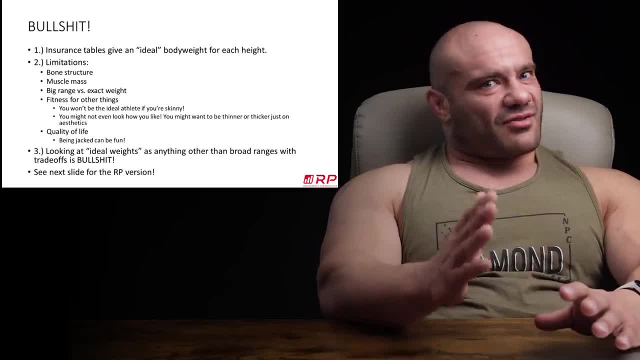 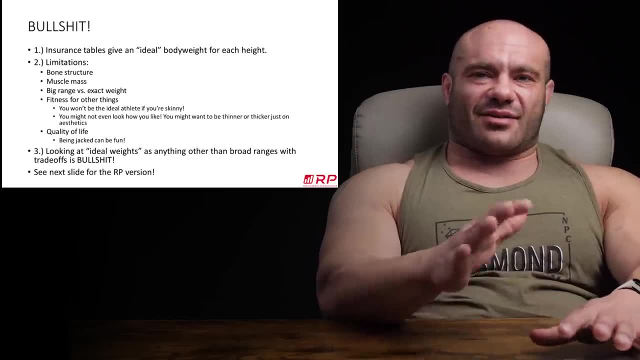 healthy weight tells you Skinnier than average, unless you get really skinny, it's not bad for your health. So if you really like the thin aesthetic, like I think it's sweet, you know I want to look like a fucking strung out, like. 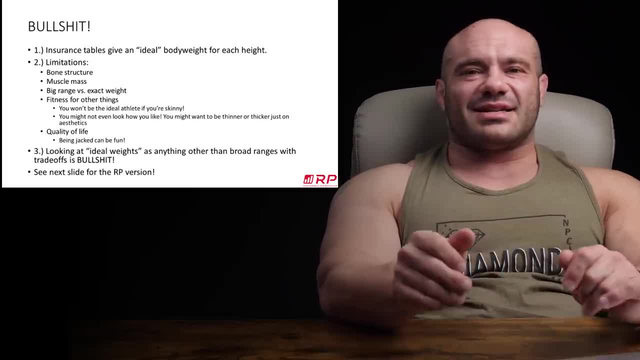 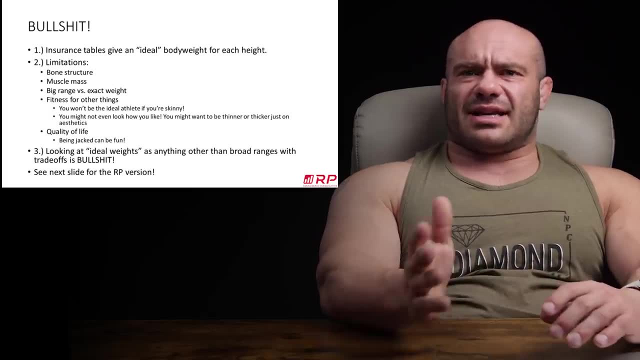 Japanese anime character. Like if the metaverse turns out- please God, I hope it does- Then, like I'll have an avatar like where I'm skinny as fuck. It'll be kind of cool. That's totally a thing you can do- And like a lot of people- and skinny people put up with the shit all the time. 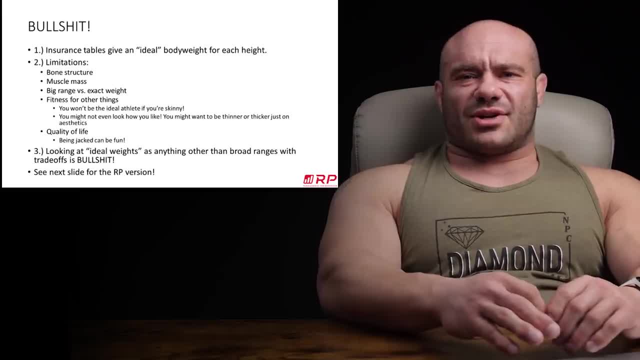 although they're skinny, it's okay. You know people would go: oh, you're thin and bones, you're skin and bones, you should eat Like motherfucker. I'm fine, My health is fine. I don't want to eat any more than I feel like. Sometimes people are just skinny and that's. 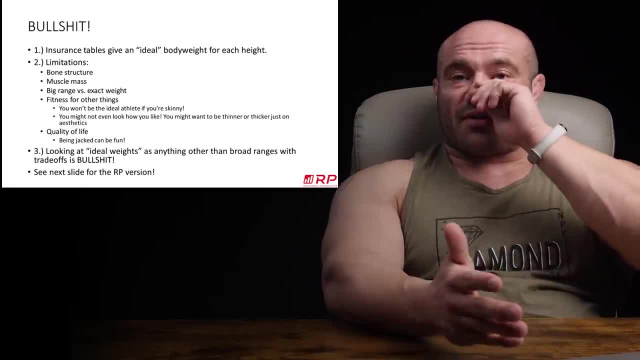 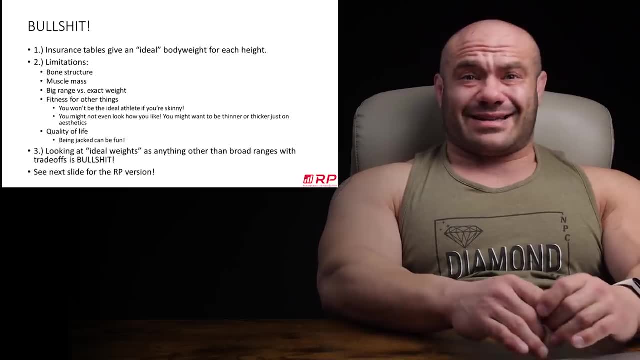 okay And that's what they want to look like. Aesthetics never enters the equation. What about thicker people? Like, first of all, muscular people And the second of all like, for example, there's a ton of girls out there that rock that thickness? God damn, they look good And they. 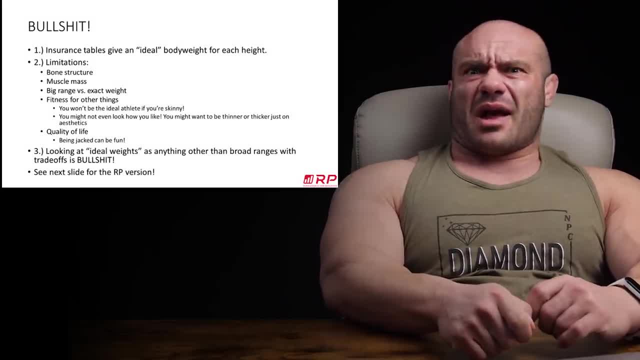 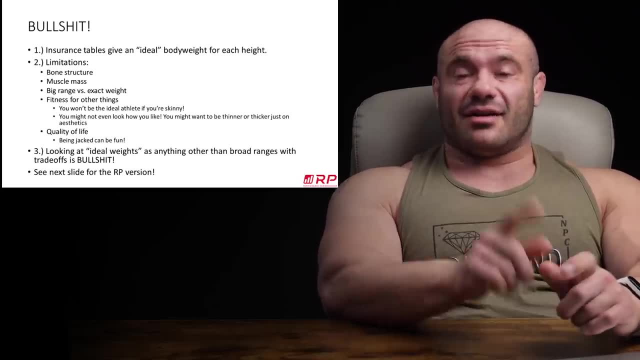 know they look good And that's how they want to look. And then someone's like: um, you're like 20 pounds overweight for your ideal weight. I'm saying: girl, you're looking pretty ideal to me. Insert your name here. My wife Crystal. Ah, yes, you brought that shit back. I'm not hitting. 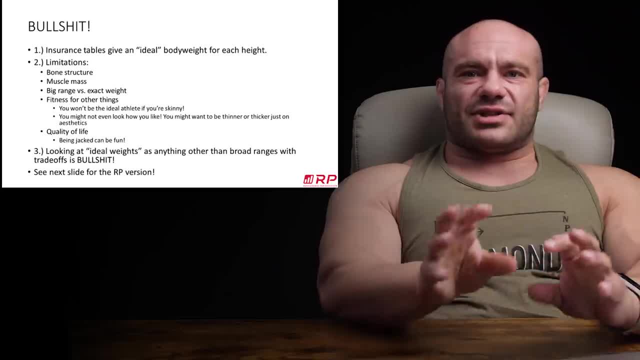 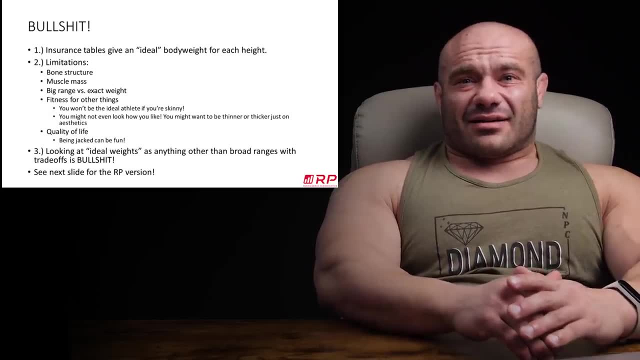 on imaginary girls on YouTube, after all. So there's a lot of considerations in there. I'll tell you what the last one is: quality of life. Being jacked is fun, Like, yeah, you could be on the beach and some guy of ideal weight comes up to you and he's like: 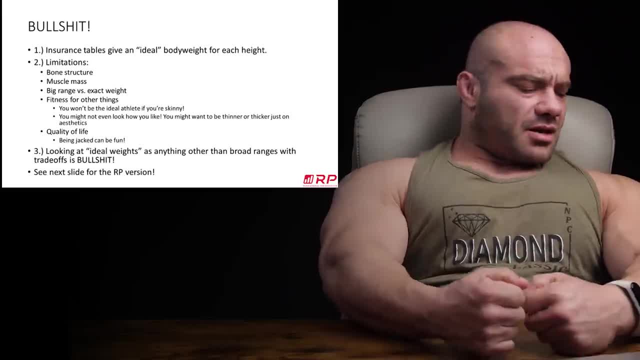 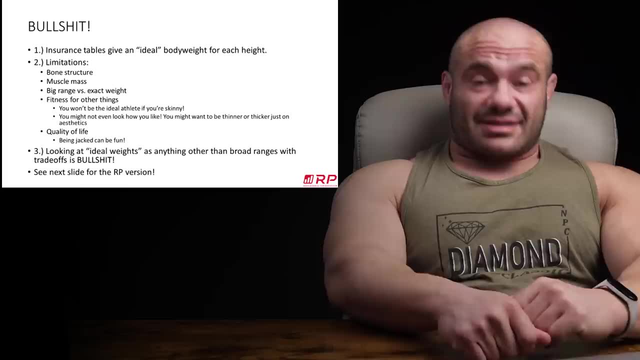 you using that space over there for your picnic blanket And you get up and you're like motherfucker, I'm using all the space. I'm like a fucking quantum non-locality. I'm in your shit at the same time. Fuck out of here And the Harry Potter scamper their way off. 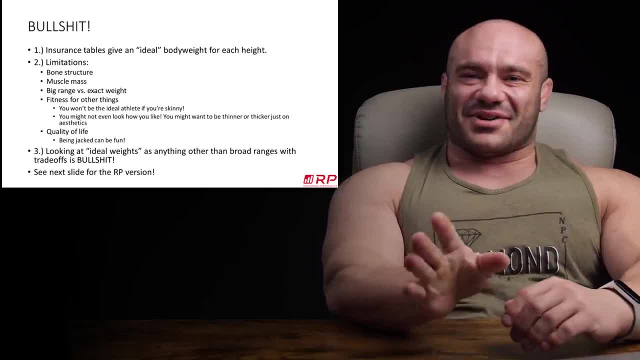 Intimidation isn't the only reason you'd want to be jacked, but God damn, it's a good one. I'm totally kidding. So, yeah, quality of life like being jacked is the shit, And as long as you're. not crazy far off. you're not going to be jacked. And if you're jacked, you're going to be jacked. And if you're jacked, you're going to be jacked. And if you're jacked, you're going to be jacked. 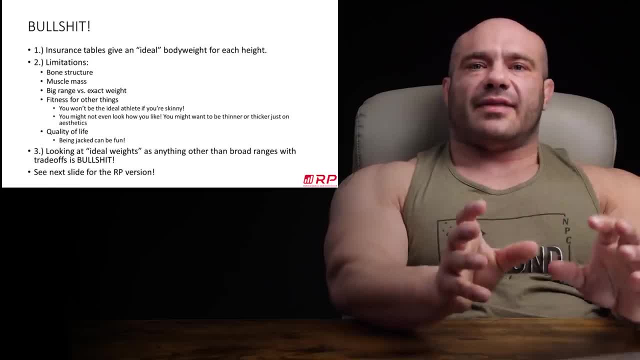 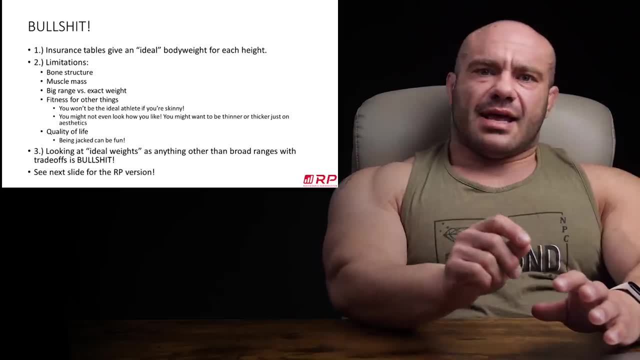 And if you're not out of that healthy range, a lot of being jacked is well within that normal range. So the idea that you look at this just one ideal weight for your height and think that's what I have to weigh and anything else is a bad idea is bullshit, as Arnold would no doubt say. And 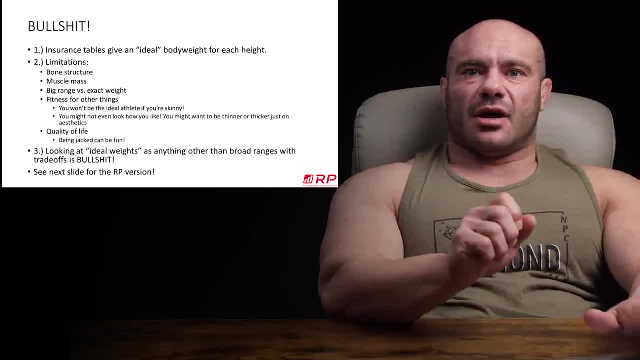 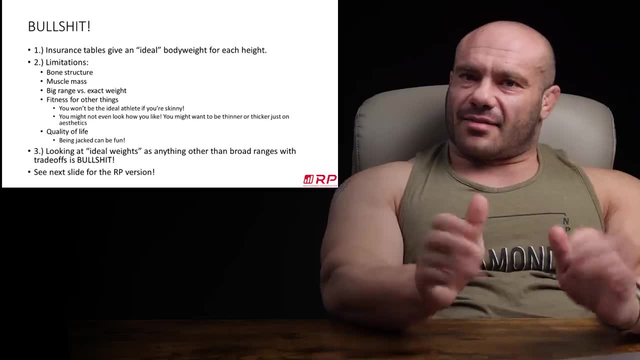 let's take a look really quick. We have the RP expanded version from one of our books. The book is, by the way, called Understanding Healthy Eating. It is available for sale if you're into paying me money. Remember, Lamborghinis don't actually self-assemble and you don't pick them like you. 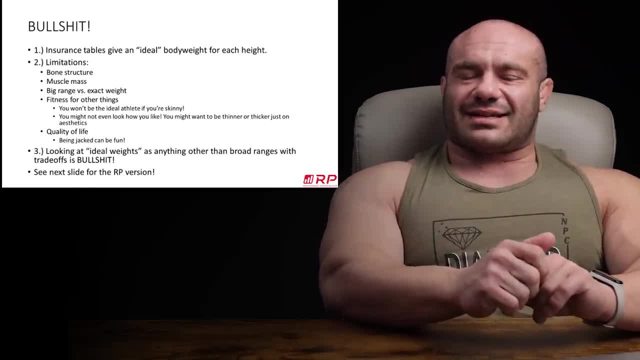 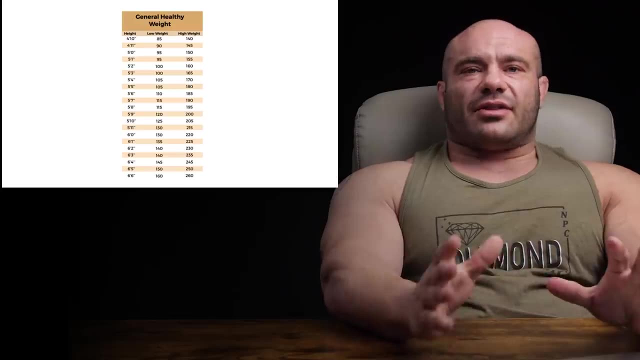 do fruits. They're built in a factory by very, very highly qualified technicians and they cost money, And I want them, more of them. So please buy my books. I don't want to beg, but I'll beg, Please, please. In any case, the you guys see it right there. general healthy weight range. 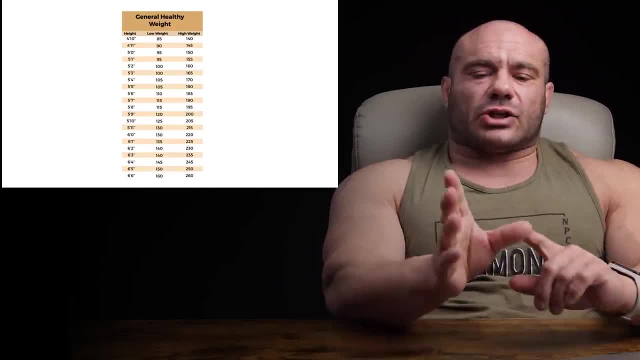 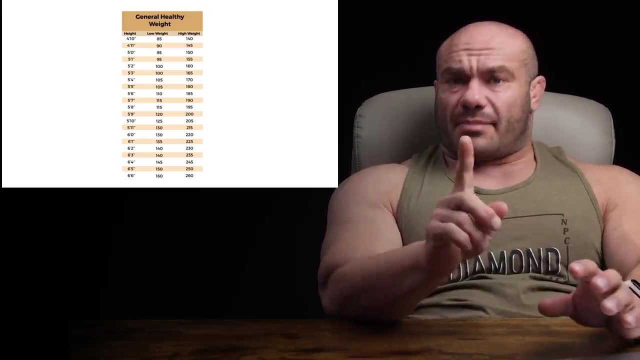 for any given height is actually really big As long as you're physically active, eating mostly healthy foods. if you're in this range, any show up to a doctor, a competent doctor's office. there's no reason for them to tell you: hey, you should think about gaining. 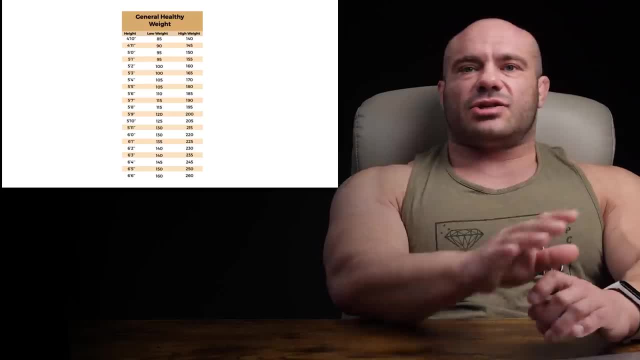 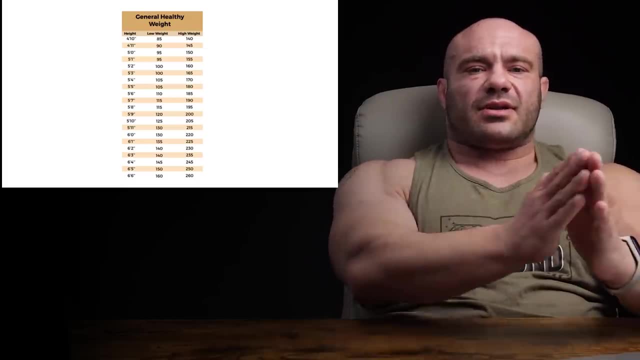 weight or you should think about losing weight, Any one of these. when you're within this range, you're totally good. As long as your blood work is good and you're physically active and you're eating healthy, your weight is not an issue And what you choose to be within that range is. 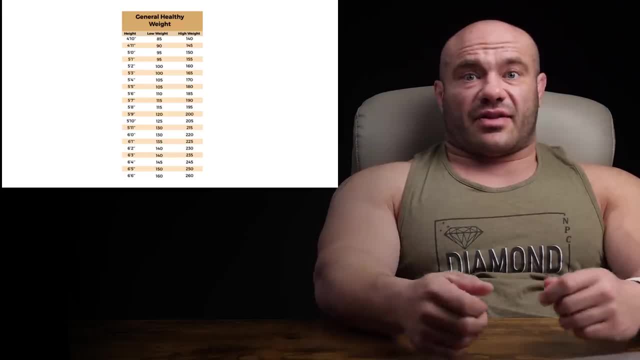 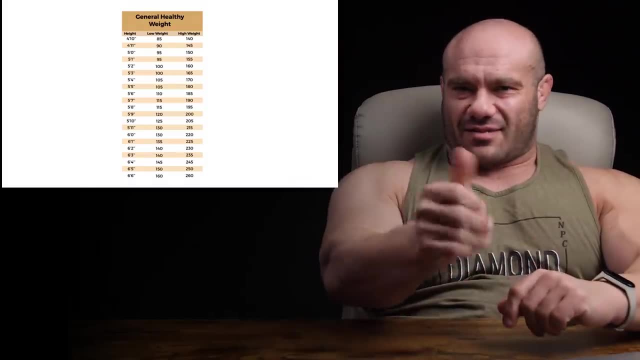 entirely up to, just like how you want to live your life for the next little bit. You want to be thick as fuck and get you know what I'm saying. Get on the club and pop that shit and have motherfuckers be like: oh, I've been, I've seen movies about clubs before. Or you want to 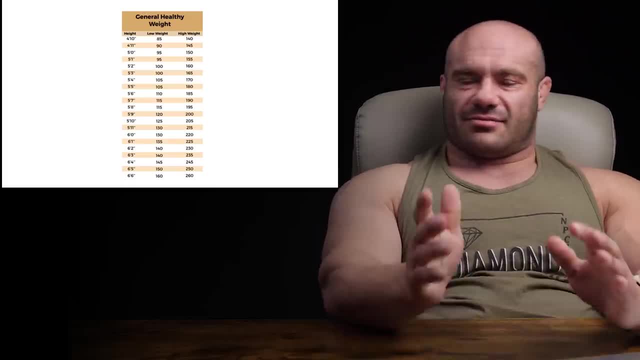 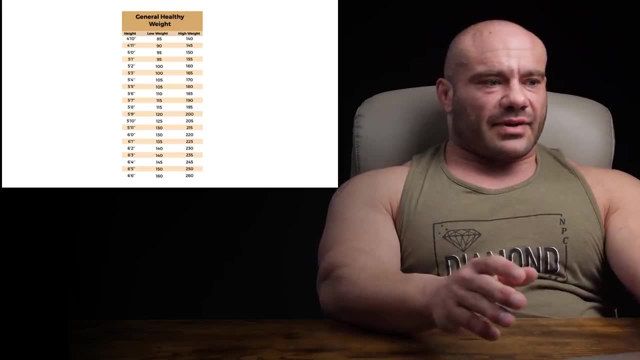 if I can rock that Kate Moss swag, that cocaine chic, all good. Well, if you use cocaine, your health will deprecate to some extent, But in any case there's a lot of right answers to what I'm trying to say. So, for example, you know, let's say you're a female, allegedly 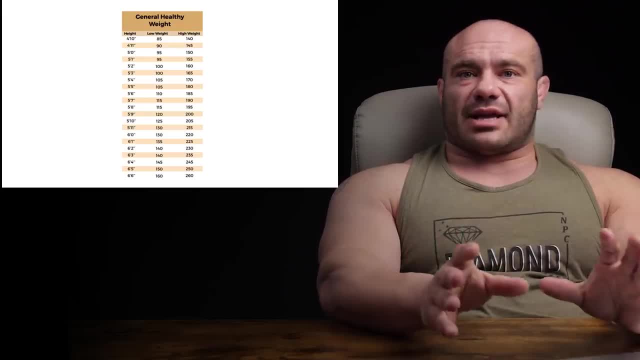 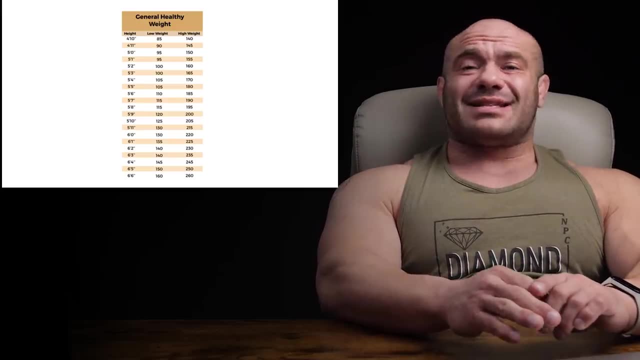 hypothetically and you're a five foot four, what is potentially a healthy weight? The weight range here is 105 pounds to 170 pounds. Five foot four- 170 is thicker than fuck. God damn what up baby. But on a serious note, 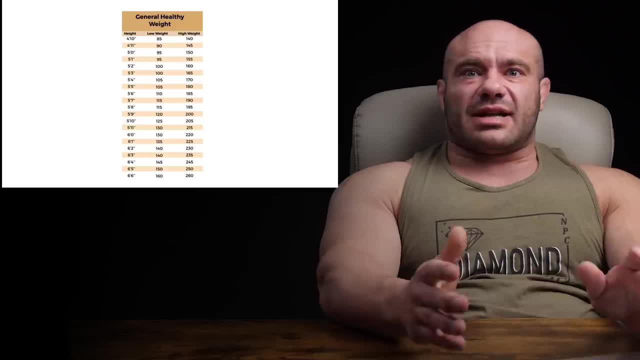 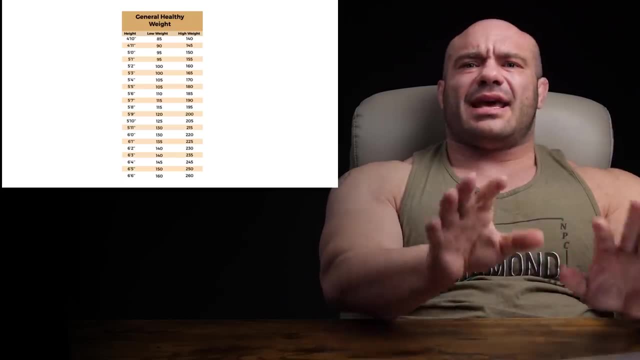 105 pounds at five four is like, yeah, you're pretty thin, but none of these are dangerous. They're not bad for you. This whole range, as long as you're physically active and you're eating mostly healthy foods, you can be at peak health in anything between these two And the idea that 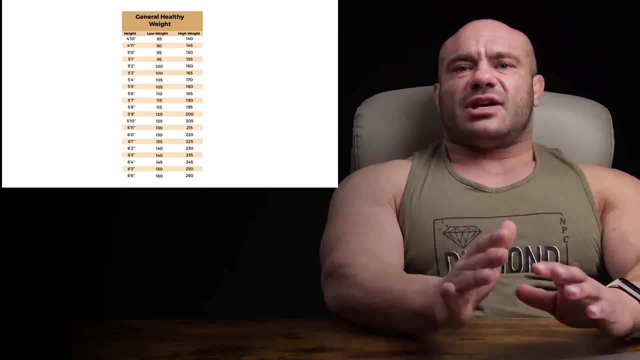 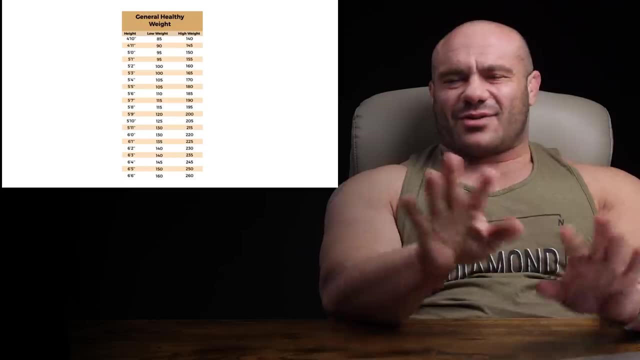 like only 120 pounds for someone who's five, four is the right weight range is just not true. It's bullshit. I really lazily did the Arnold voice on that one. Lastly, real, quick, real. this video's over, Video's over. You can click off at this point. Hold on, I'm five, six, Let's see what the 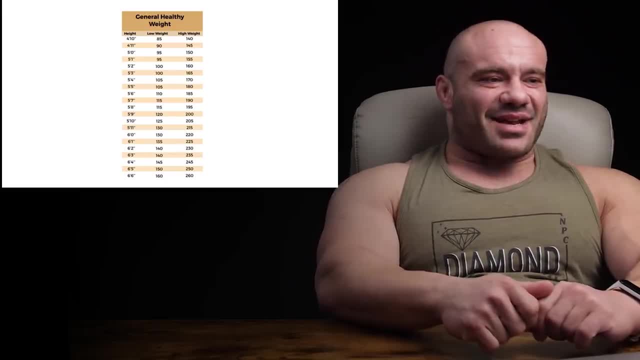 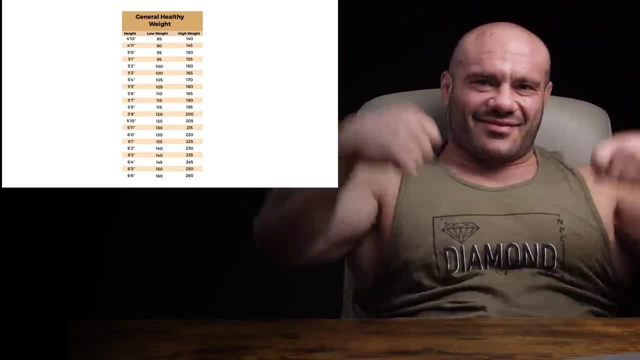 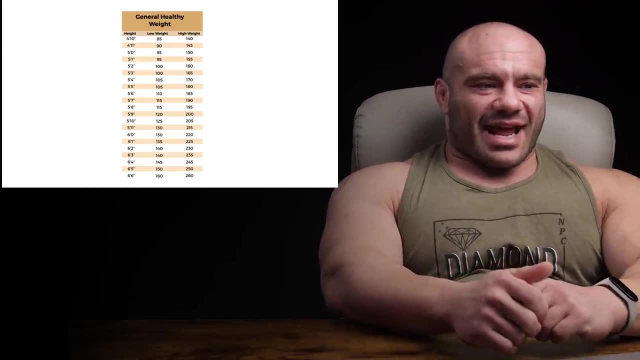 249 pounds. by the way, Yeah, Yeah, Hell yeah. How's the lighting Scott video guy? Do I look jacked? And it tops out at 185 pounds. Okay, Which begs the question: am I in the healthy weight? 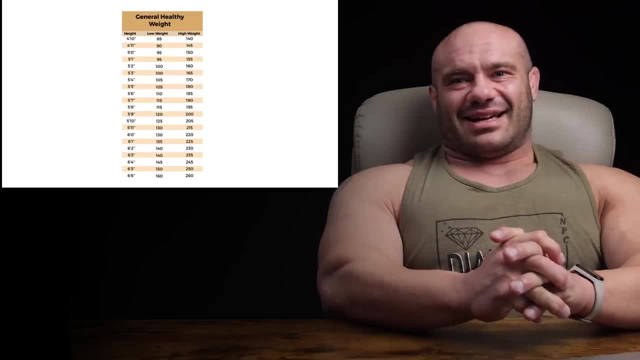 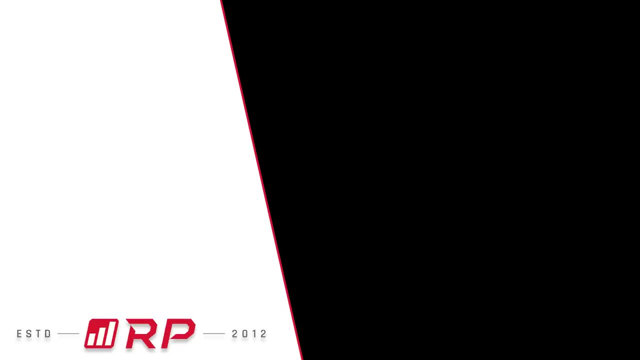 range. No, no, I'm not, I'm worried now. See you guys next time. See you next time.